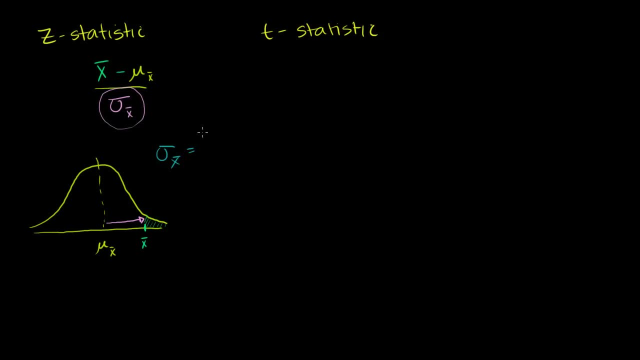 thing right here. this thing is going to be the same thing as the sample, is going to be the same thing as the standard deviation of our population, the standard deviation of our population divided by the square root of our sample size. So this thing right over here can be rewritten as our sample. 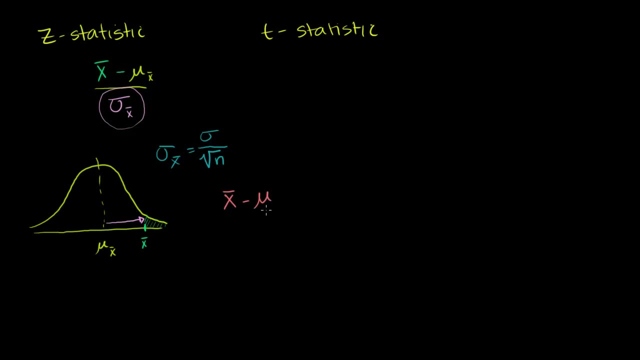 mean minus the mean of our sample size. OK, So this is the mean of our sampling distribution of the sample mean divided by this thing right here, Divided by our population, mean divided by the square root of our sample size. And this is essentially our best sense of how many standard. 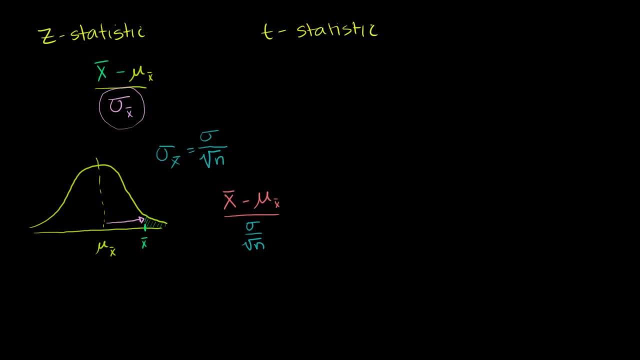 deviations away from the actual mean we are. And this thing right here, we've learned it before- is a z-score. Or when we're dealing with an actual statistic, when it's derived from the sample mean statistic, we call this a z. 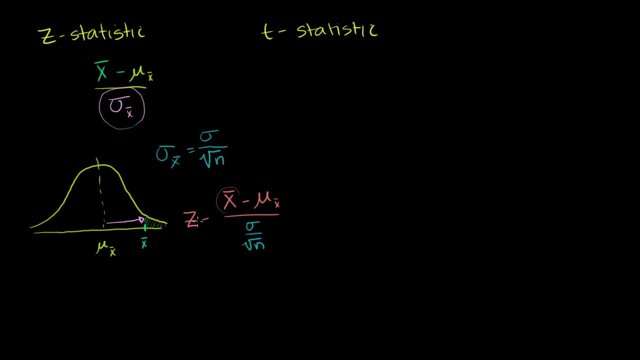 statistic And then we could look it up in a z-table or in a normal distribution table to say what's the probability of getting a value of this z or greater. So that would give us that probability. So what's the probability of getting that? 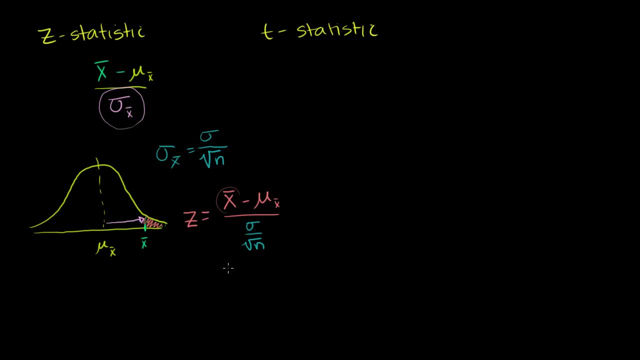 extreme of a result. Now, normally, when we've done this in the last few videos, we also do not know what the standard deviation of the population is. So, in order to approximate that, in order to approximate that, we say that the z-score is approximately, or the z. 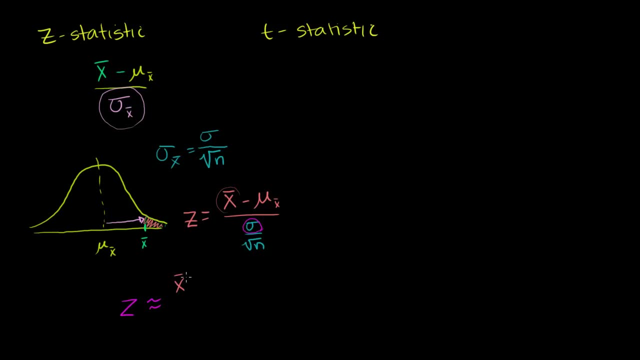 statistic is approximately going to be, so let me just write the numerator over again over. we estimate this using our sample standard deviation. We estimate it using our. let me do this in a new color with using our sample standard deviation, using our sample. 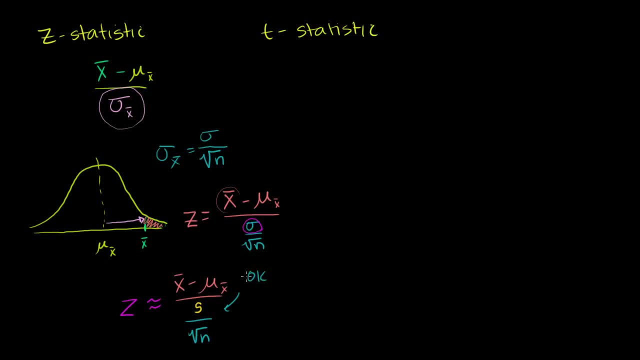 standard deviation And this is OK. This is OK. OK If our sample size is greater than 30. Or another way to think about it is: this will be normally distributed if our sample size is greater than 30. Even this approximation will be approximately. 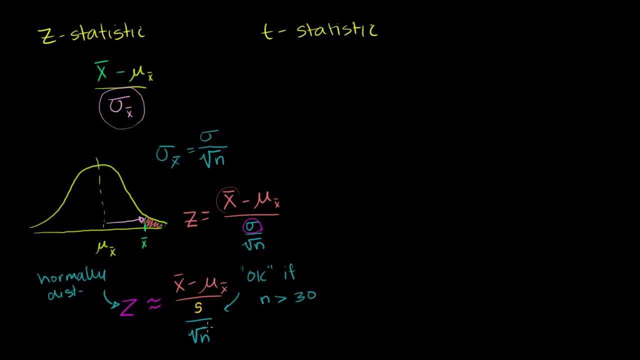 normally distributed. Now, if your sample size is less than 30, especially- it's a good bit- less than 30,, all of a sudden this expression will not be normally distributed. So let me rewrite the expression over here. Sample mean minus the mean of your sampling. distribution of 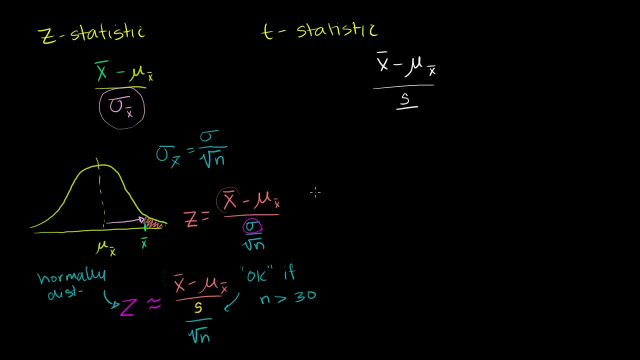 the sample mean divided by your sample standard deviation over the square root of your sample size. We just said, if this thing is well over 30, or at least 30,, then this value, right here, this statistic is going to be. 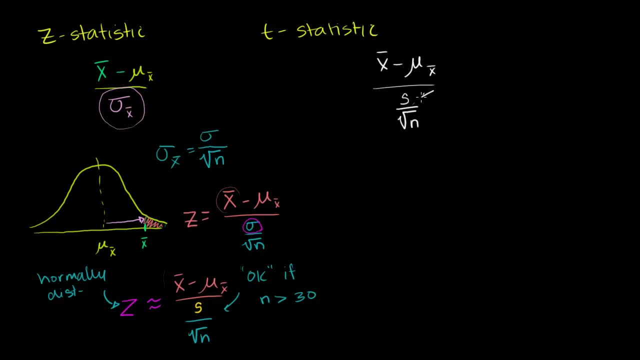 normally distributed. If it's not, if this is small, if that is small, then this is going to have a t distribution, This is going to have a t distribution, And then you're going to do the exact same thing you did here. 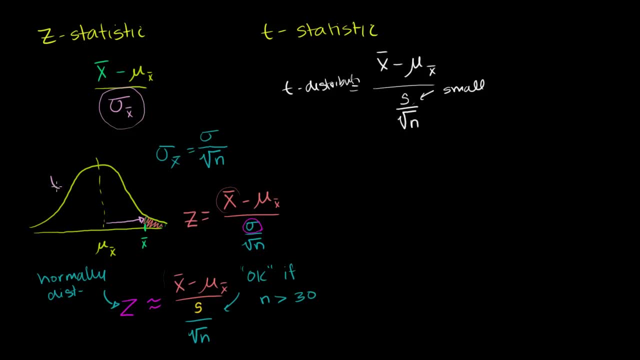 but now you would assume that the bell is no longer a normal distribution. So in this example it was normal. It was normal. All of the z's are normally distributed Over here in a t distribution and this will actually be a normalized t distribution right here, because we subtracted out. 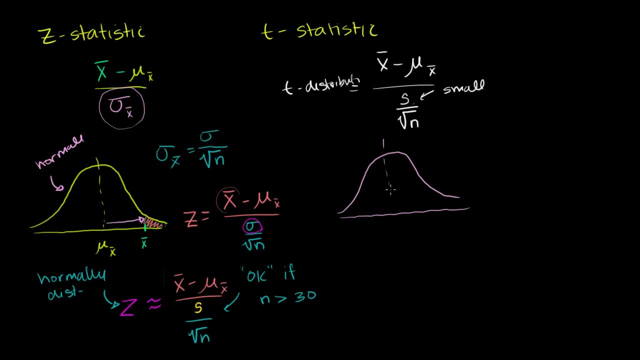 the mean. So in a t distribution, in a normalized t distribution, you're going to have a mean of 0. And what you're going to do is you want to figure out the probability of getting a t. You want to figure out the t value, at least this extreme. 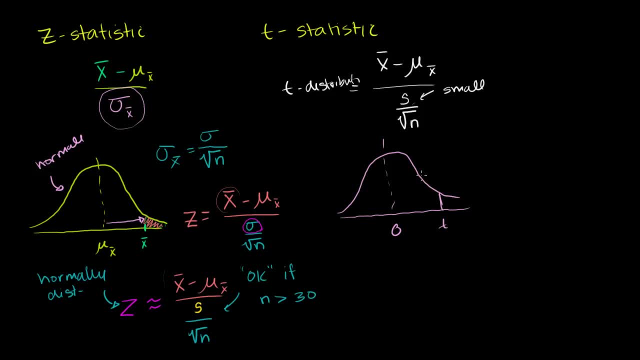 So this is your t value you would get, And then you essentially figure out the area under the curve right over there, And so a very easy rule of thumb is: calculate this quantity either way. If you have more than 30 samples, if your sample size is, 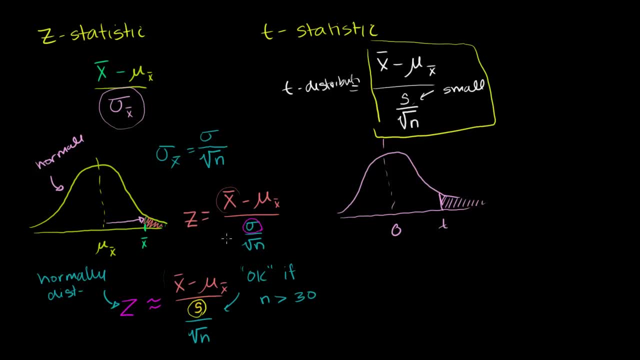 more than 30, your sample standard deviation is going to be a good approximator For your population standard deviation, And so this whole thing is going to be approximately normally distributed, And so you can use a z table to figure out the probability of 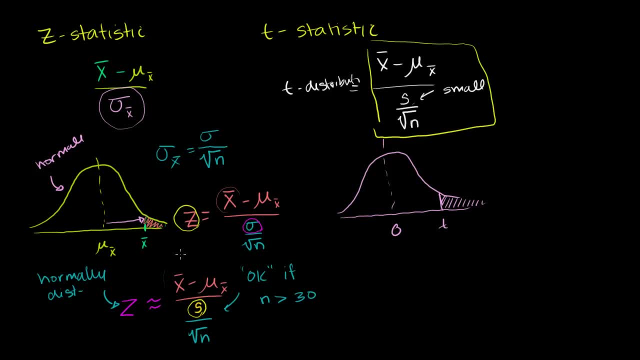 getting a result at least that extreme. If your sample size is small, then this statistic, this quantity, this is going to have a t distribution And then you're going to have to use a t table to figure out the probability of getting a t value at least this extreme.